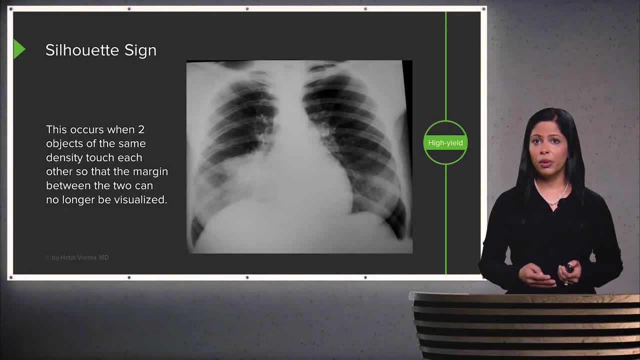 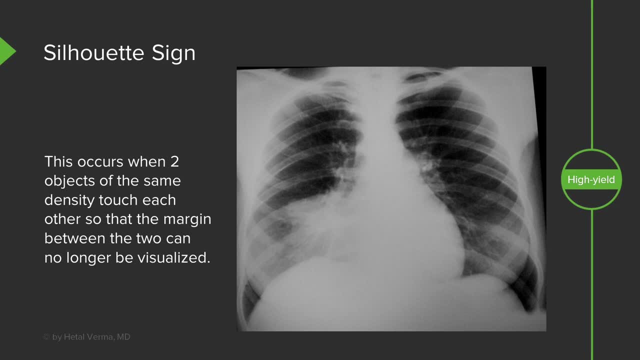 This was briefly mentioned in one of our introductory lectures and it's a very common radiological sign. It occurs when two objects of the same density touch each other so that the margin between the two can no longer be visualized. So if you look here, there's an area of consolidation involving the right middle. 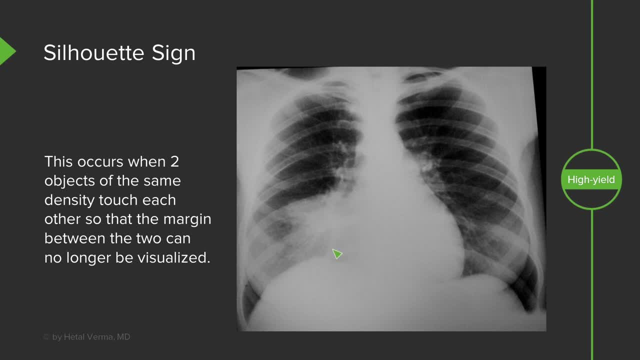 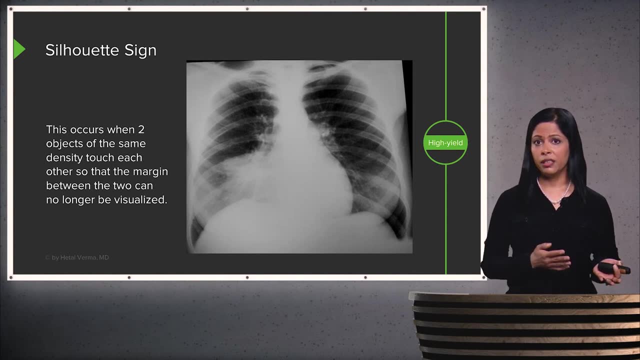 lobe and you can see that the right heart border is no longer visible. So the area of consolidation is silhouetting the right heart. And again this occurs because the consolidation is of equal density to the heart, and now you can no longer see the margins between the two. 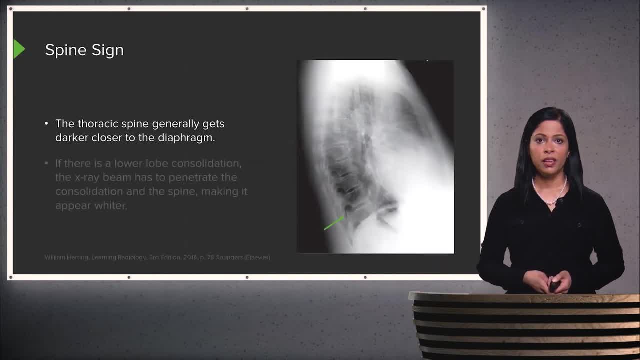 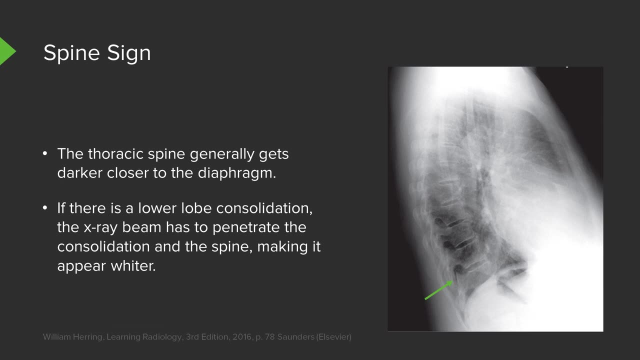 The spine sign is another sign that we can see with consolidation. So in general, the thoracic spine gets darker as we get closer to the diaphragm. However, if there is a lower lobe consolidation, the x-ray beam has to penetrate the consolidation and the spine, making it appear wider. 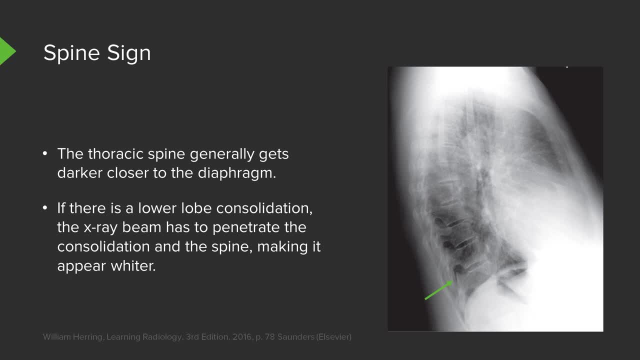 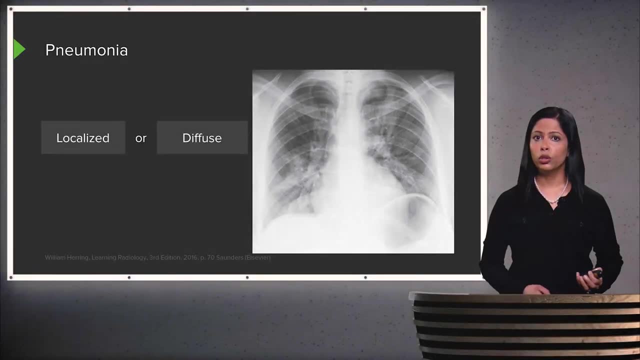 So this is an example of summation of shadow. So when you have multiple shadows overlapping each other, the area appears wider than you would normally expect. So pneumonia can be either localized or diffuse. It can also be airspace or interstitial, So there are a variety of different ways that pneumonia can present, and pneumonia is one of the most common causes of consolidation. 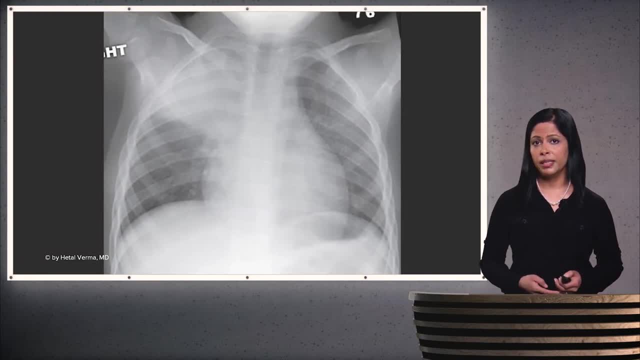 So let's go over some signs of pneumonia and some patterns that we may see. So these patterns are important to kind of keep in your mind because they come up relatively often And then you can see what the pattern represents. So let's take a look at this frontal chest x-ray. 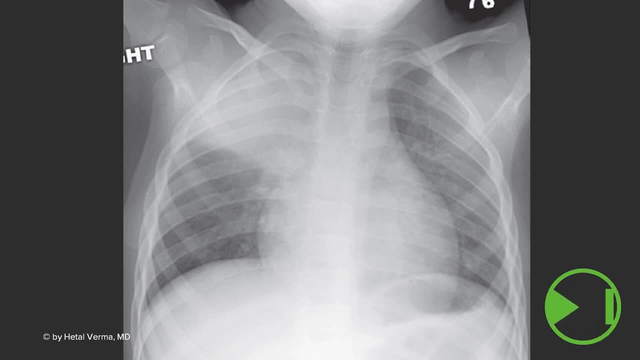 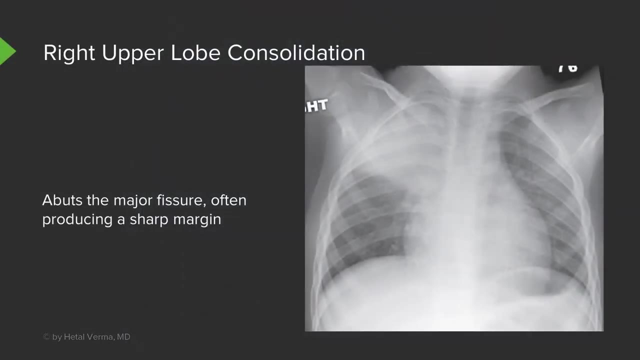 What do you see here? And as we go through this lecture, feel free to pause and take a good look at the images. So this is an example of right upper lobe consolidation. The consolidation abuts the major fissure which produces a sharp margin inferiorly here. 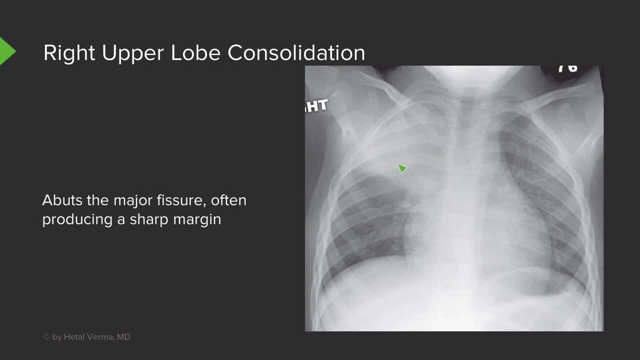 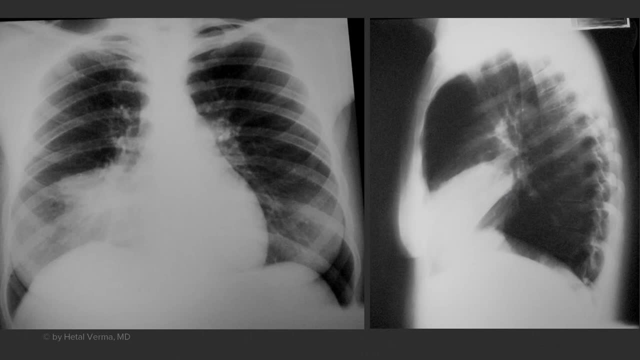 And it involves the entire right upper lobe. You can see that it silhouettes the mediastinum, The mediastinum on the right. So where do you think this consolidation is located? We have a frontal and a lateral view in a patient that's presenting, let's say, with cough. 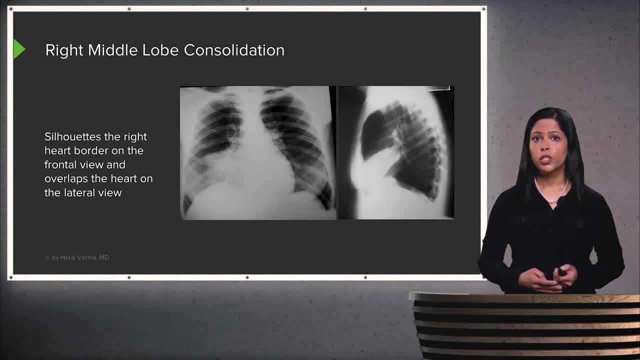 So this is an example of right middle lobe consolidation. So on the frontal view, the right heart border is silhouetted so that we don't see it anymore, And on the lateral view, a middle lobe consolidation will overlap the heart. 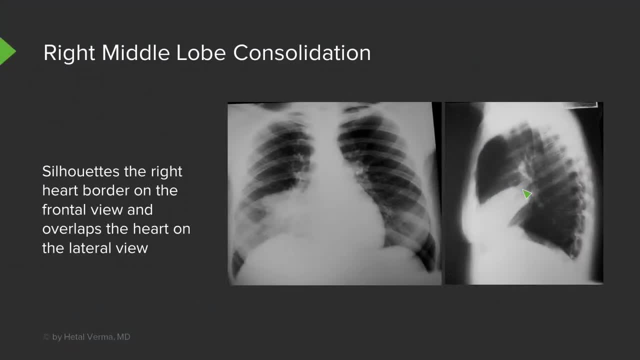 So if you look here, the heart appears brighter than it normally would, And that's because this consolidation that you see on the frontal view is located adjacent to the heart, anteriorly on the lateral view, And this is very typical of a right middle lobe consolidation. 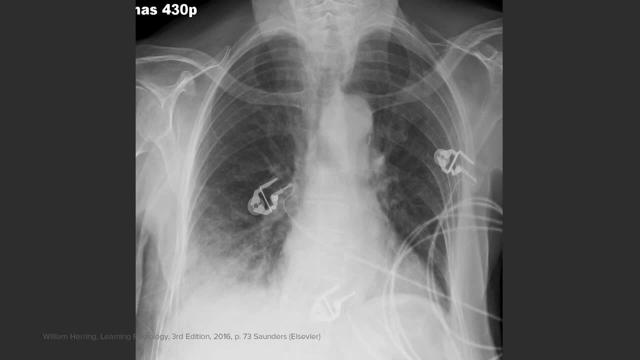 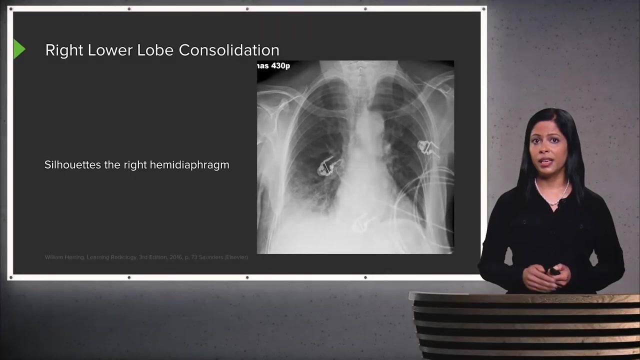 Let's take a look at this pattern. So this patient is also presenting with a consolidation. Where do you think this consolidation is located? Which part of the lung do you think it's in? So we have silhouetting of the right hemidiaphragm. 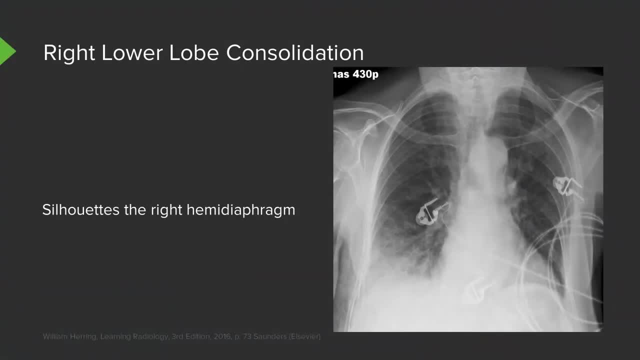 This is what a right lower lobe consolidation would look like. So remember to differentiate between a right middle lobe consolidation and a right lower lobe consolidation. on a frontal view, the right middle lobe consolidation will silhouette the right heart border, while the right lower lobe consolidation will silhouette the right hemidiaphragm. 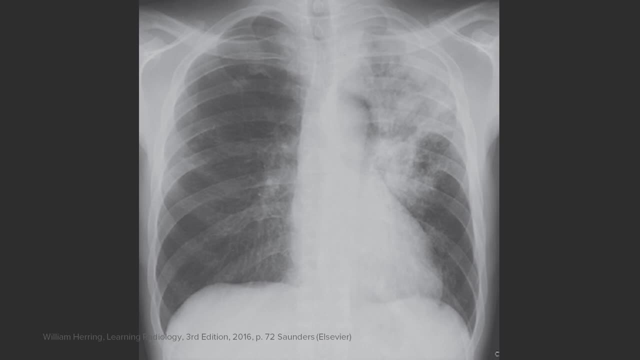 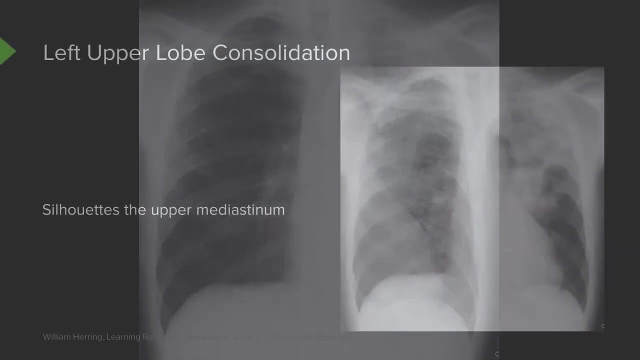 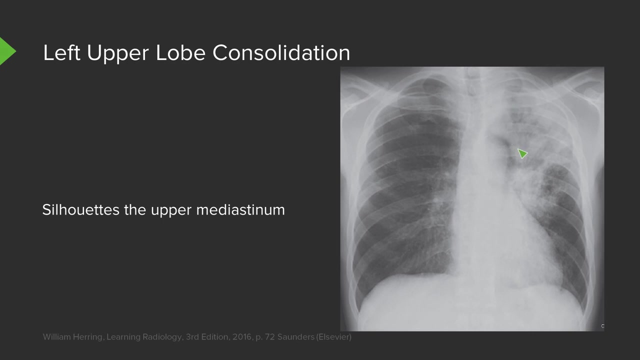 How about this chest x-ray? Where do you think this consolidation is located? So this is an example of a left upper lobe consolidation which again silhouettes the left side of the upper mediastinum. In this one you can actually see some of the classic signs of air bronchograms. 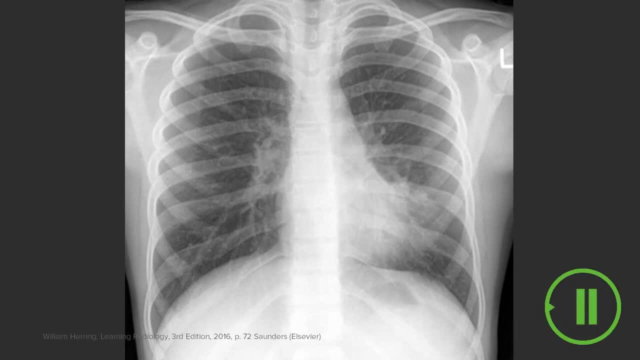 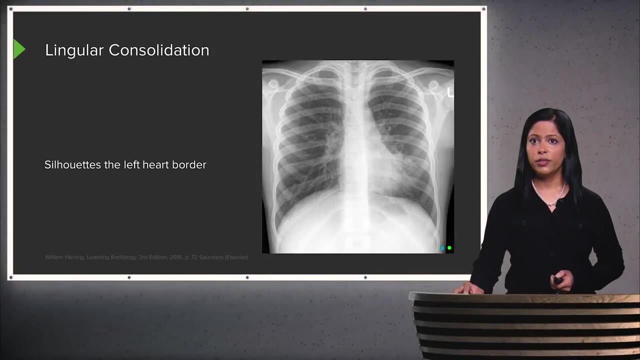 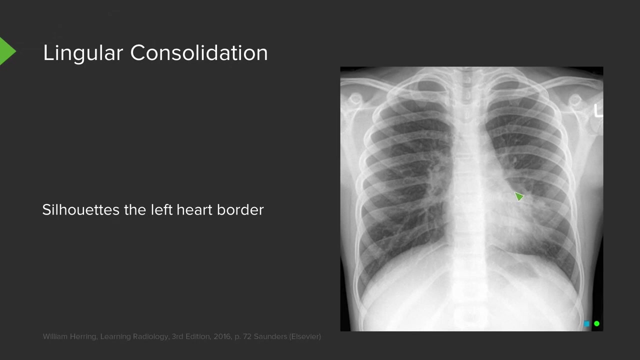 And what do you see on this one? So here we have silhouetting of the left heart border. You can see that the right heart border is pretty clearly visualized, while the left heart border has a sharp margin here and then all of a sudden becomes somewhat hazy here. 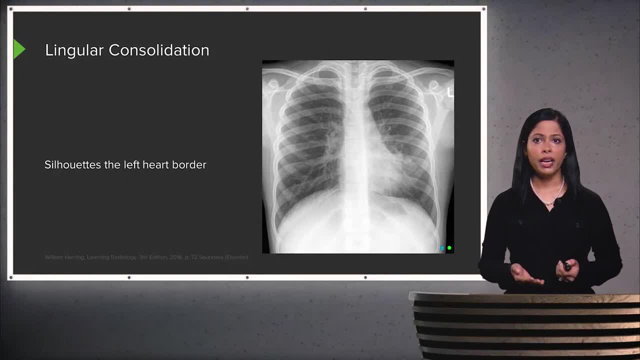 So this is an example of a lingular consolidation. So the lingula is actually a portion of the left upper lobe, if you recall. However, it's in the same location as the right middle lobe, So it's somewhat a separate structure. 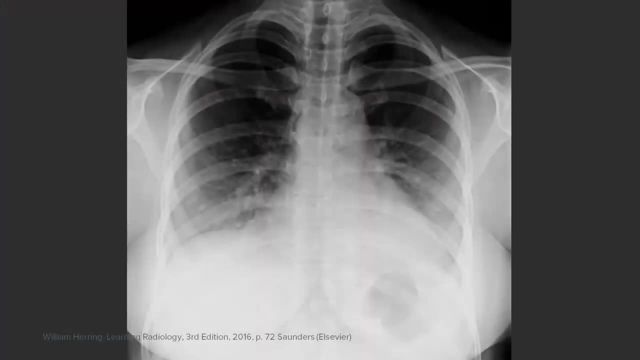 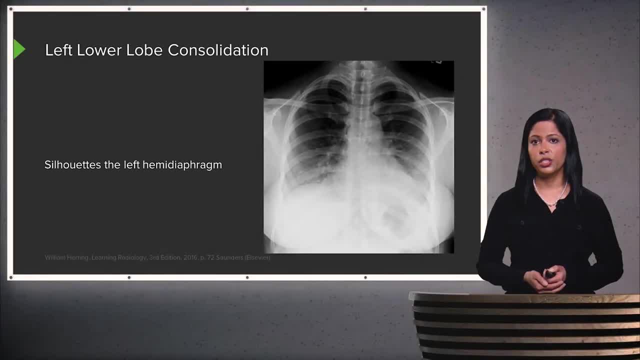 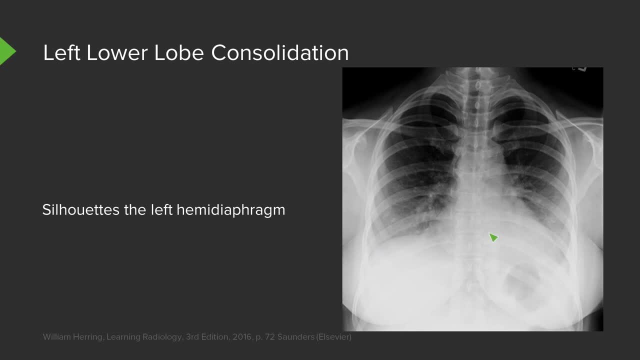 This is an example of left lower lobe consolidation. So we have silhouetting of the left hemidiaphragm here, So you can see a sharp margin here. on the right, However, the left hemidiaphragm, which is normally visualized through the heart,